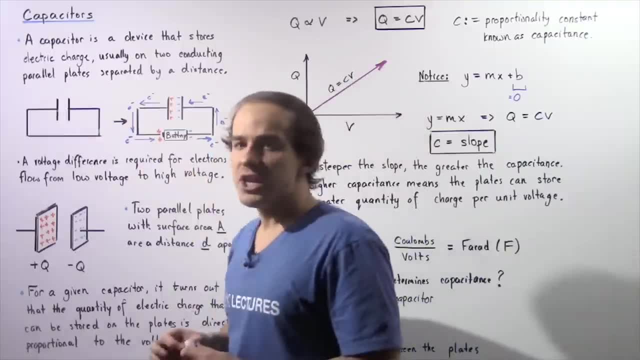 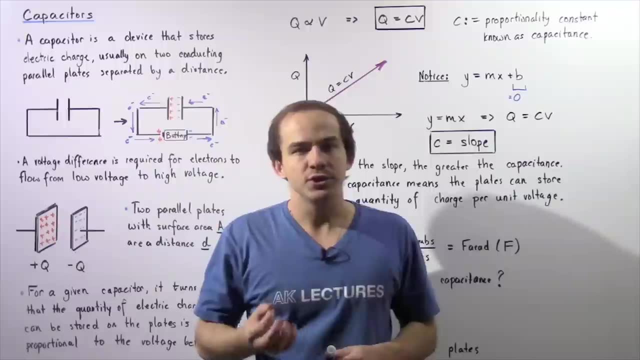 in the following diagram. Now, in this case, there is no voltage difference between plate one and plate two, and because there is no voltage difference, in other words, the voltage on plate one is even in the case of the circuit dude, the voltage on the circuit dude is even higher. And 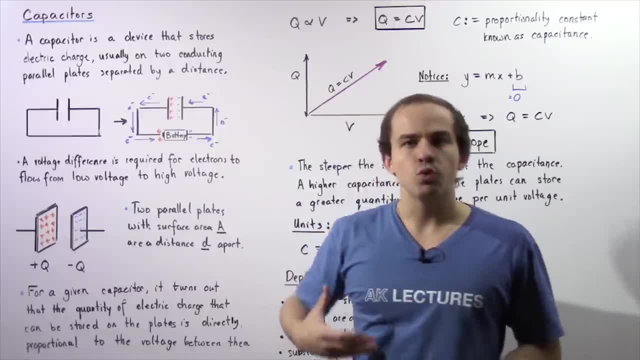 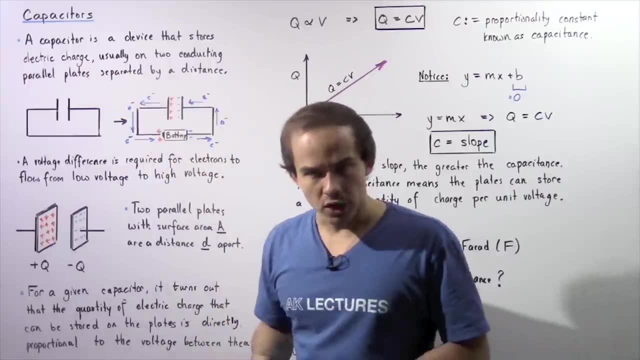 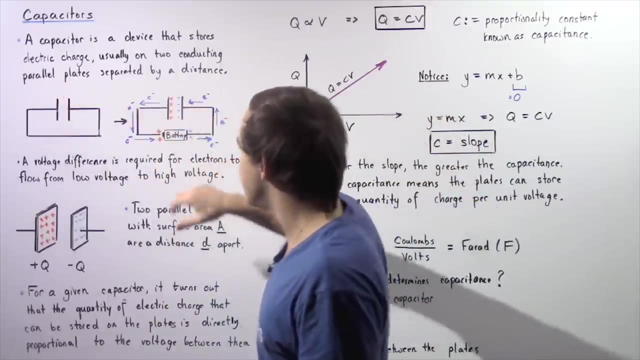 equal to the voltage on plate 2, electrons will not flow And that basically means the charges on these two plates will be neutral. Now what happens if I take a battery and I place a battery into our wire circuit, as shown in the following case? So, to go from this to this diagram, we 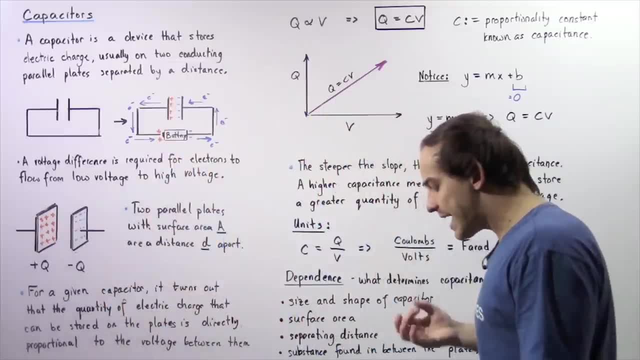 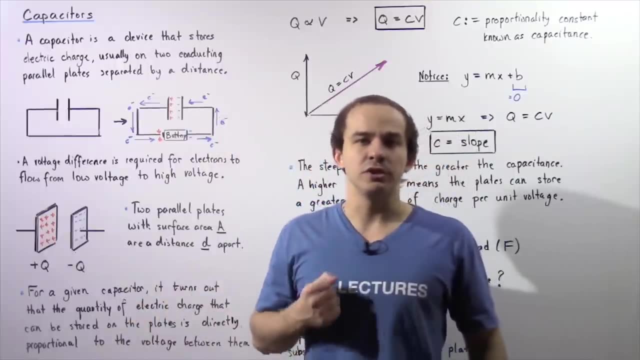 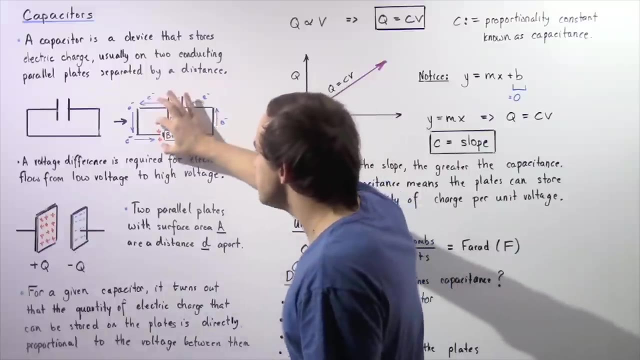 essentially insert a battery. Now, what exactly is a battery? A battery is essentially a device that creates an electric potential difference, So it creates a voltage difference. And now, because we have a voltage difference between this side and this side of our battery, electrons will begin to. 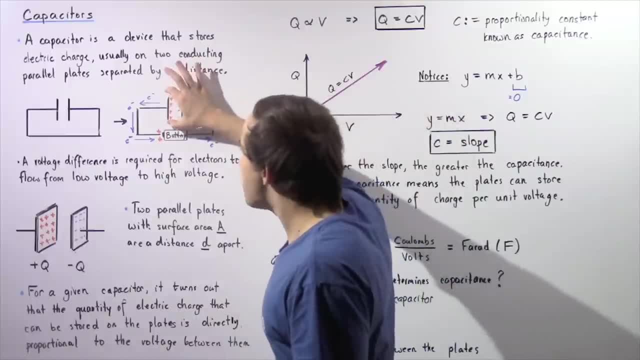 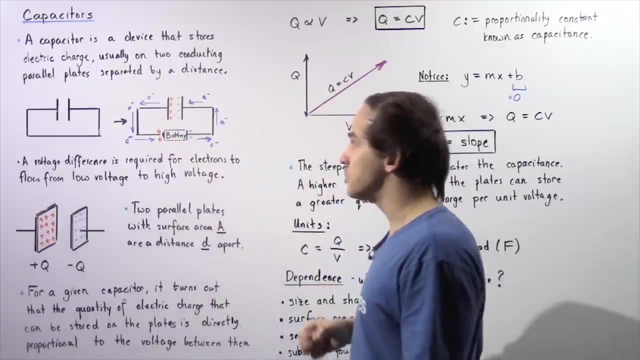 flow And electrons will flow from this parallel plate to the positive end of our battery, And electrons will flow from this parallel plate to the positive end of our battery, from a lower potential to a higher potential, and likewise electrons will begin to flow from this. 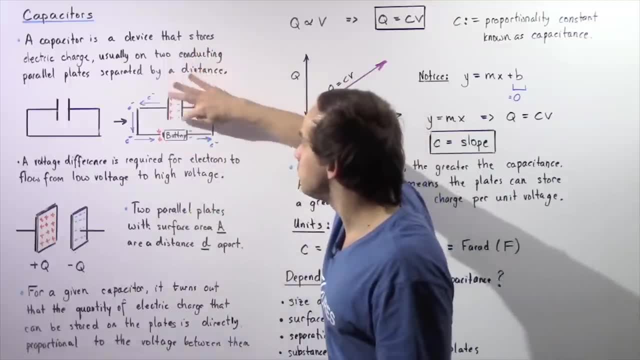 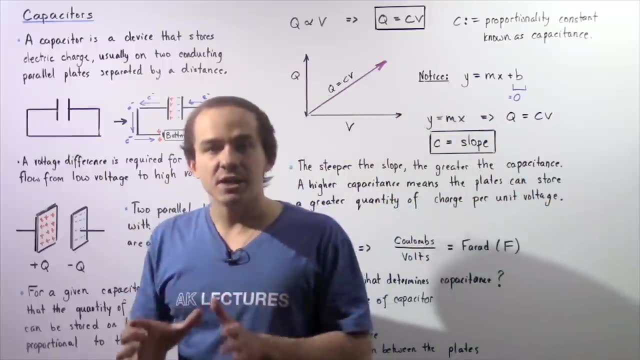 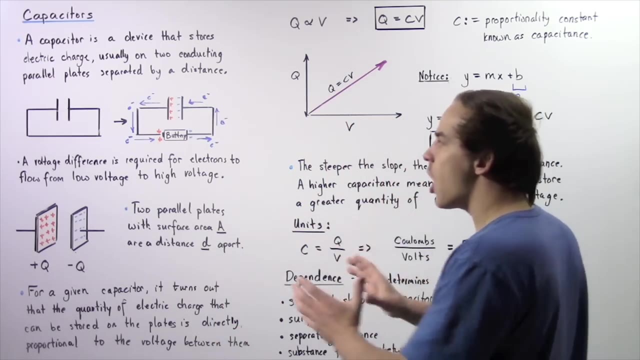 side, from a lower potential to this parallel plate to a higher potential. and now, because we have an electric potential difference, because we have a voltage difference, electrons will flow and that will create a separation of charge on these two parallel plates. so we're going to have a 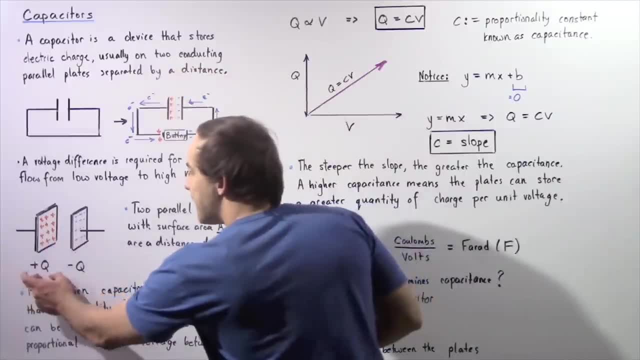 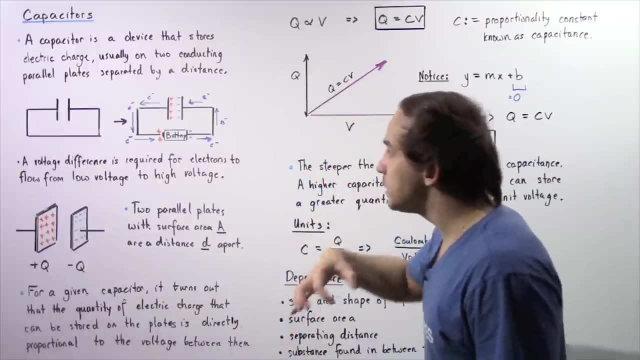 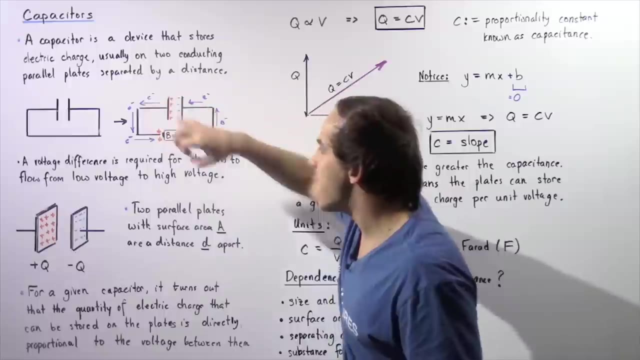 positive charge on this plate, shown here by positive q, and a negative charge on this plate, shown here by negative q. now the voltage difference between these two parallel plates will be equal to the voltage difference between these two ends of our battery. so once again, a voltage difference is required. 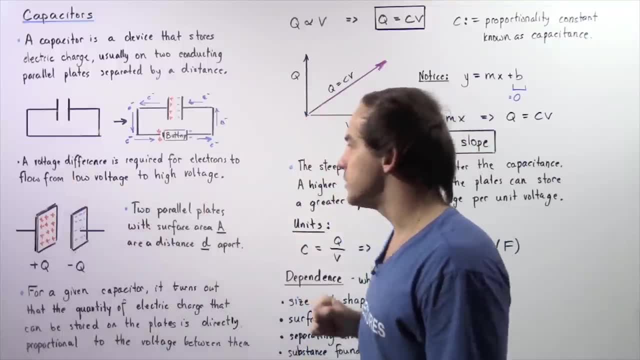 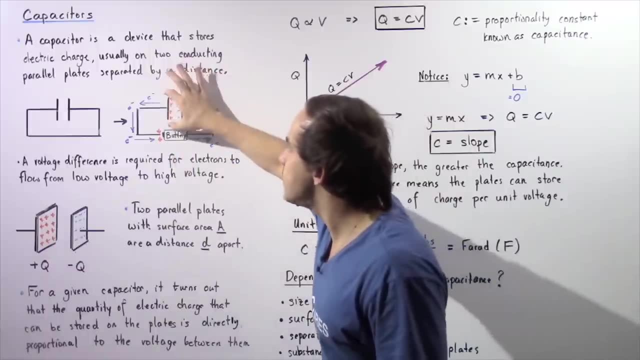 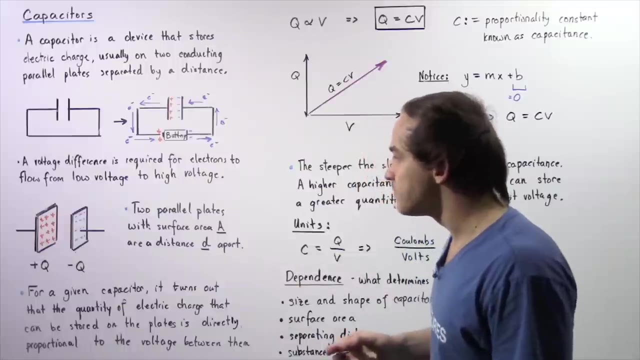 for electrons to flow from the lower voltage to the higher voltage, which is exactly why electrons collect on this plate and they leave this plate, because there is a voltage difference that exists as a result of this battery. So here we have our two parallel plates Now, these two parallel plates. 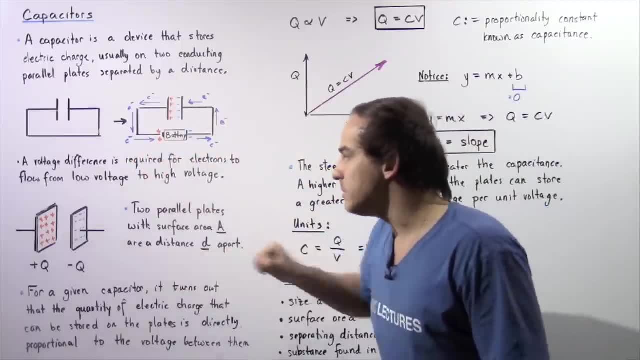 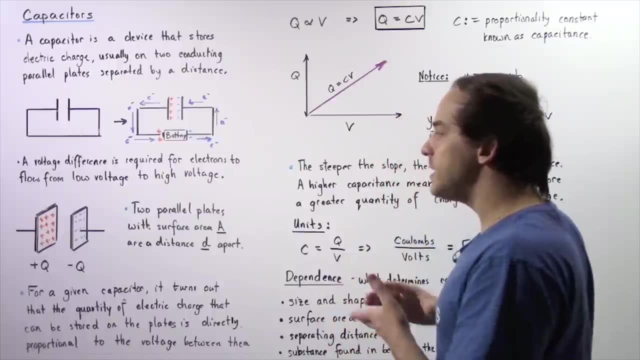 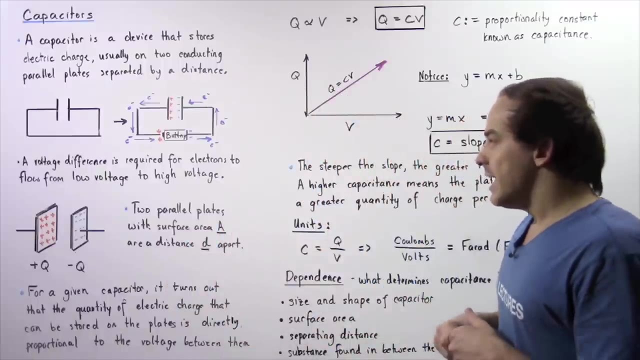 will have a surface area given by A and will be placed a certain distance- D- apart. This two quantity. these two quantities will become important when we discuss other things about capacitors in the future lectures. Now, for any given capacitor, it turns out that the quantity 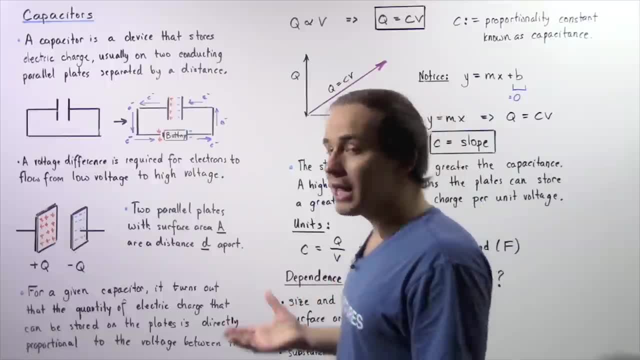 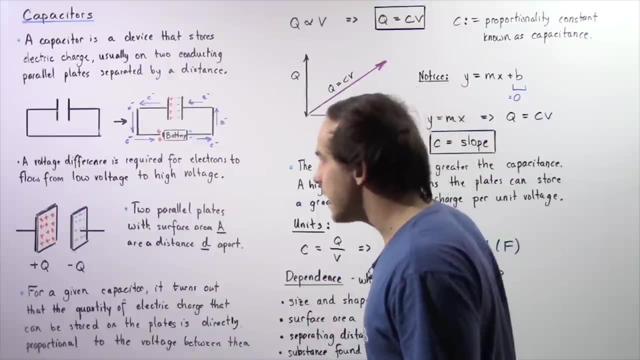 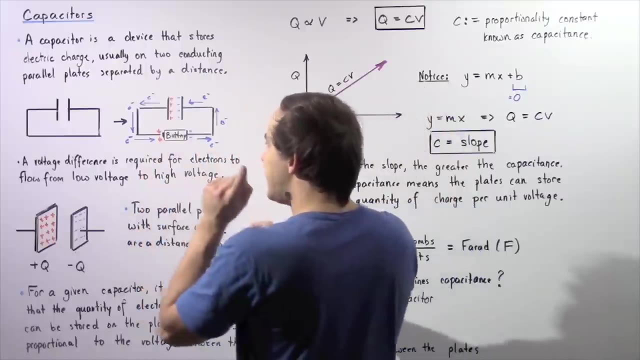 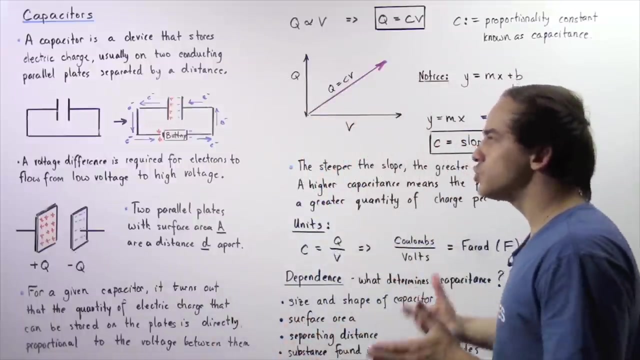 of electric charge that can be stored on these parallel plates is directly proportionate to the voltage between these two plates. So that basically means if we increase the voltage of our battery, if we increase the voltage difference that exists within our battery, the capacitors will be able to store more electric charge. So our charge is directly. 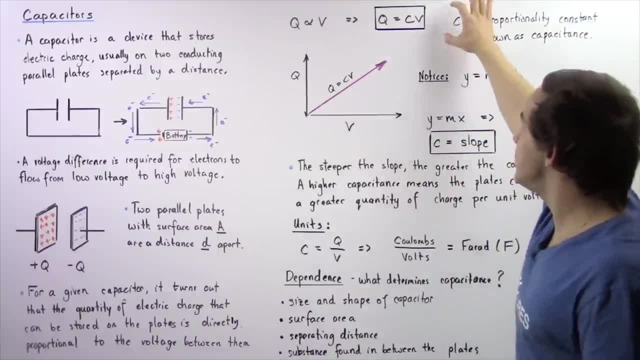 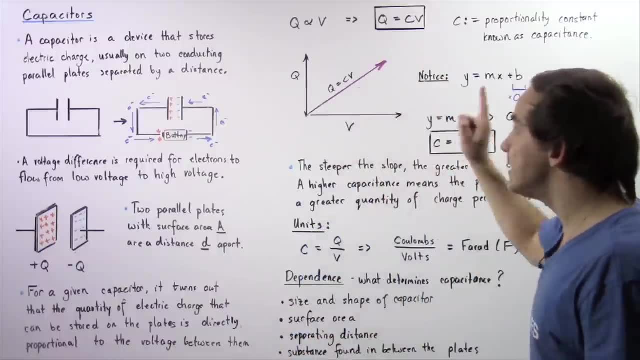 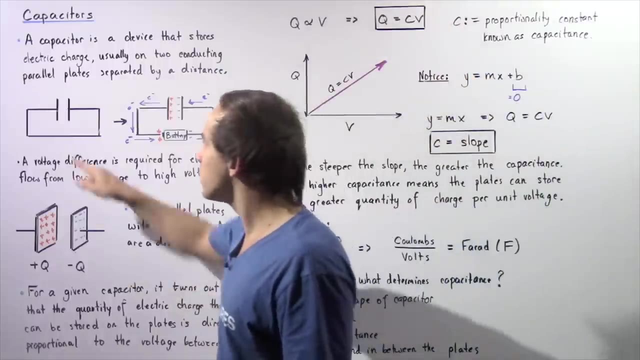 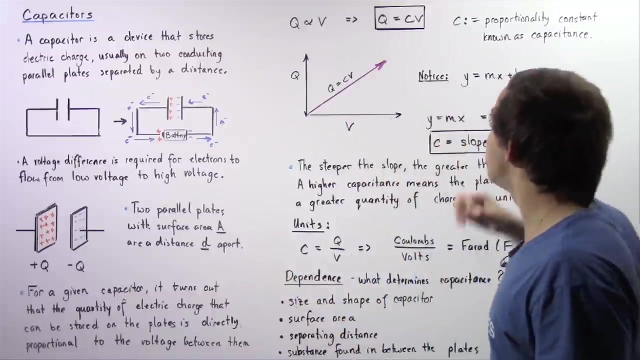 proportional to our voltage. So that basically means we have the following equation: where C is simply our voltage, Now C is also called our capacitance, So Q- the quantity of charge that can be stored on either one of these two plates, is equal to C, the capacitance of that plate multiplied by the 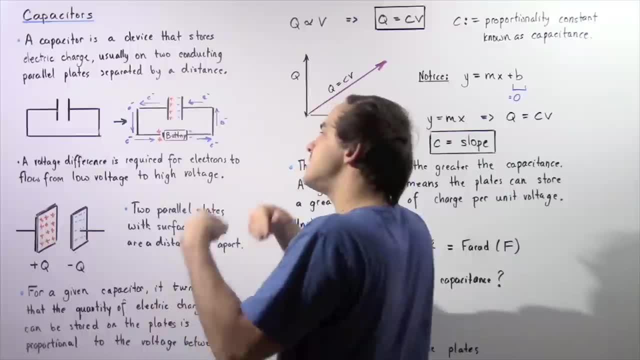 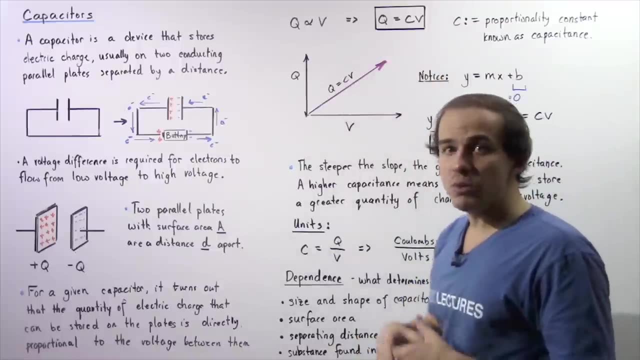 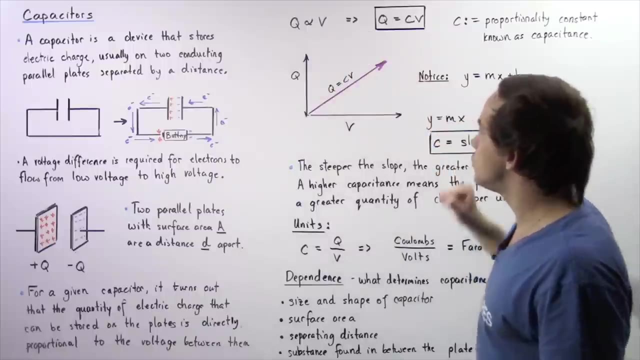 voltage difference between our battery, which is the same voltage difference that exists between our two parallel plates. So if we take this equation and we plot it on the other side of the x- y plane, we get the following linear slope: So our Q is equal to the product of C multiplied. 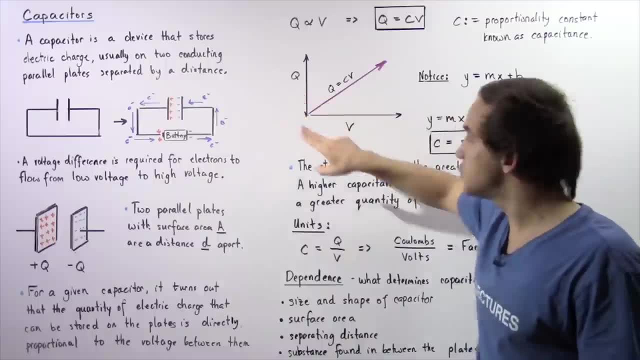 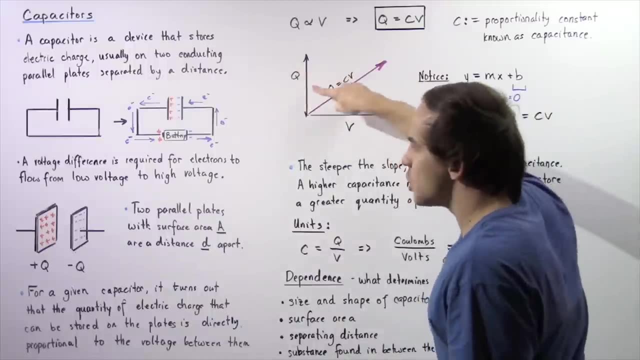 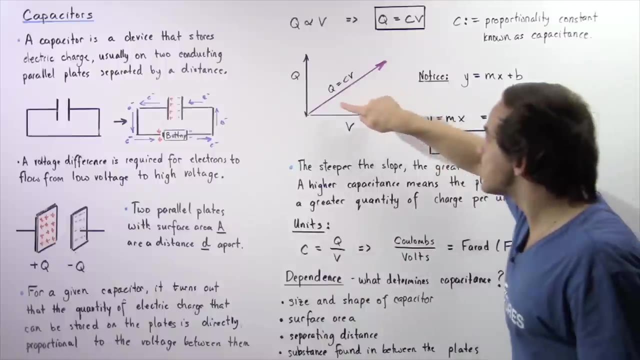 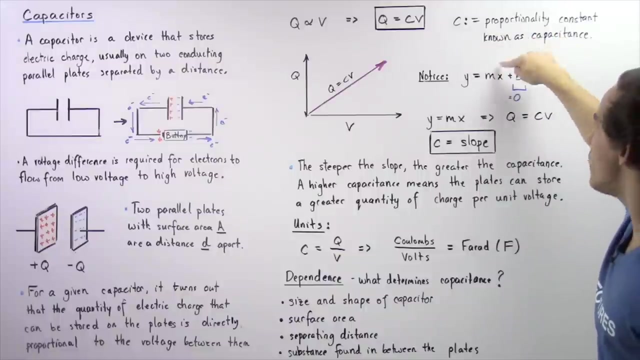 by V, where our y-axis is the charge and our x-axis is our voltage. So we see, as the voltage increases, the quantity of charge that is stored on either one of the capacitors also increases. Now notice: this is a linear equation. So y equals mx plus b, where m is our slope. 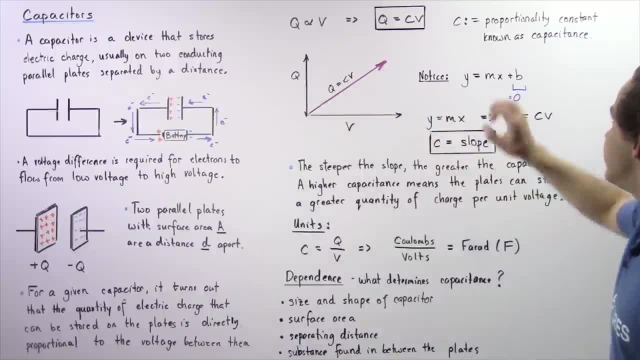 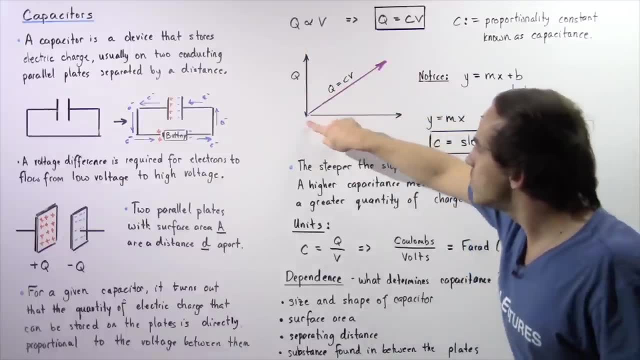 x is our x-coordinate and y is our y-coordinate and b is simply where our linear line intersects our y-axis. Now, in this case, it happens to be 0, so our b is 0, our y-intercept is 0. So that, 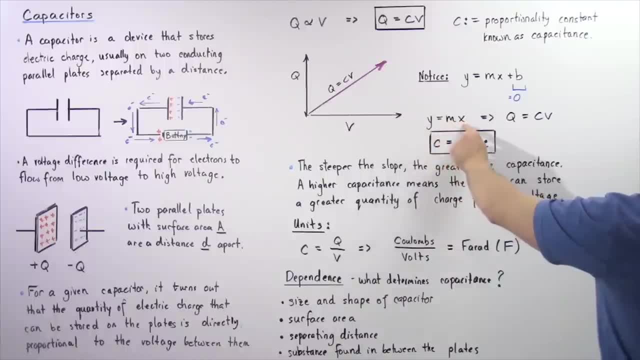 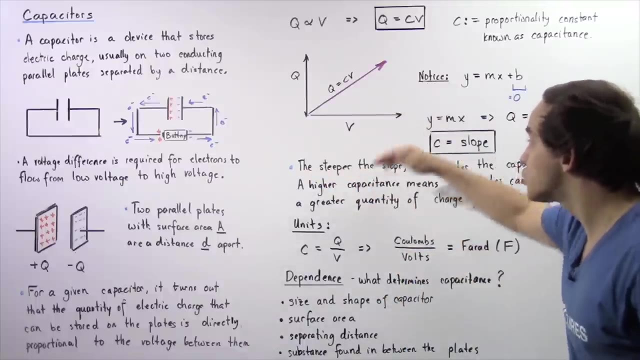 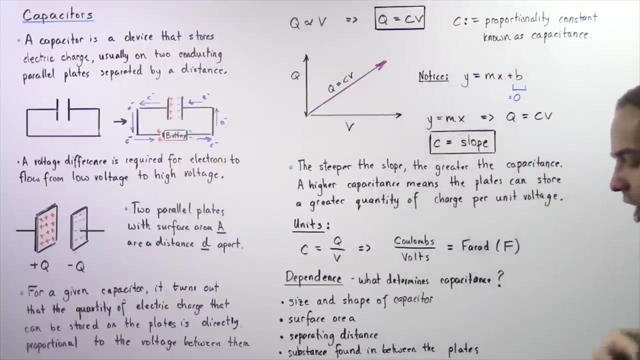 means our equation becomes: y is equal to m times x, and this is the same form as q is equal to c multiplied by v. So c is our slope, The capacitance represents our slope and we see that the steeper the slope is, the greater the capacitance is, because the greater the c value is. Now what? 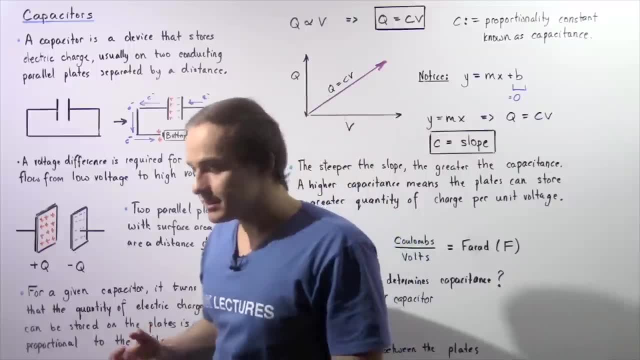 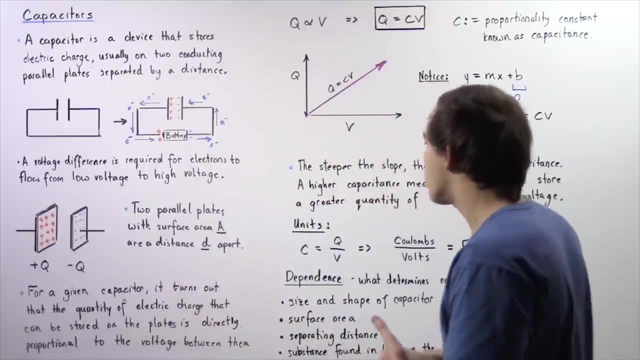 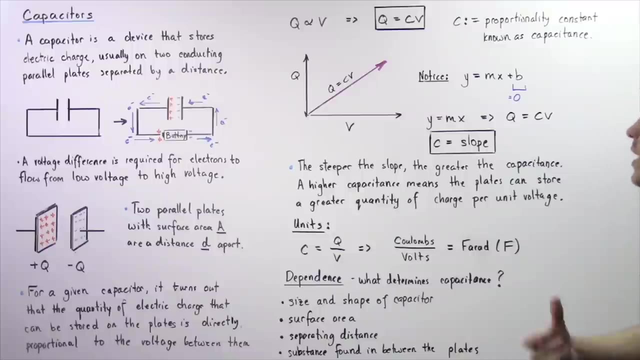 exactly is capacitance. The capacitance of any capacitor is the value of the capacitor. Capacitor is essentially how much electric charge that capacitor can store. So a higher capacitance, a higher c value means the plates can store a greater quantity of charge per unit. 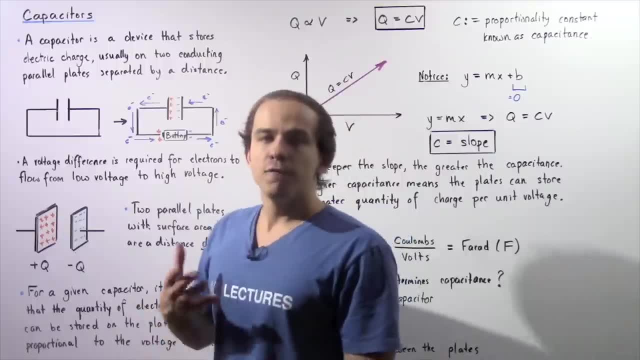 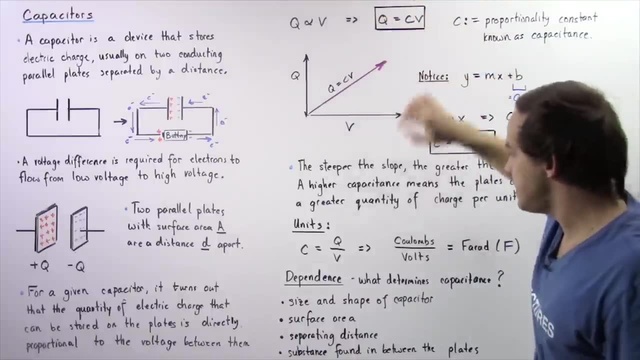 voltage. Now, what exactly are the units for capacitance? So, capacitance, we can take this equation, rearrange it and solve for our c. The capacitance given by c is the value of the capacitor. So we can take this equation, rearrange it and solve for our c. 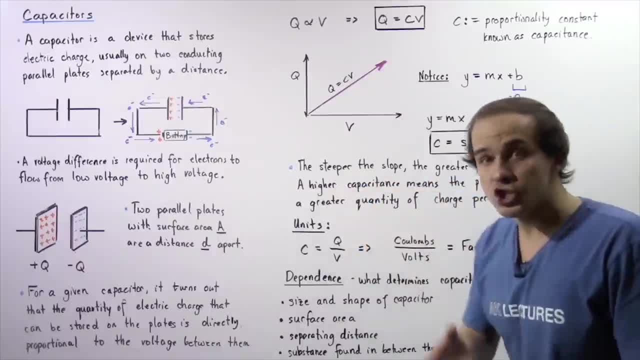 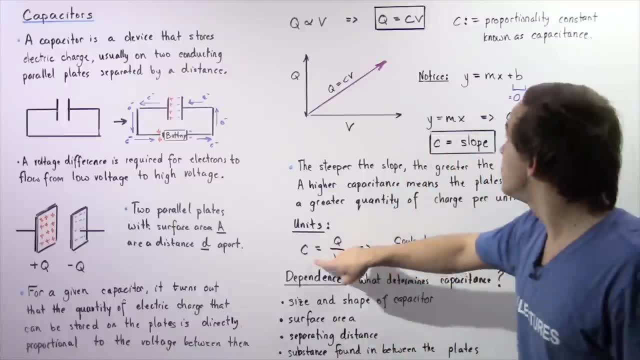 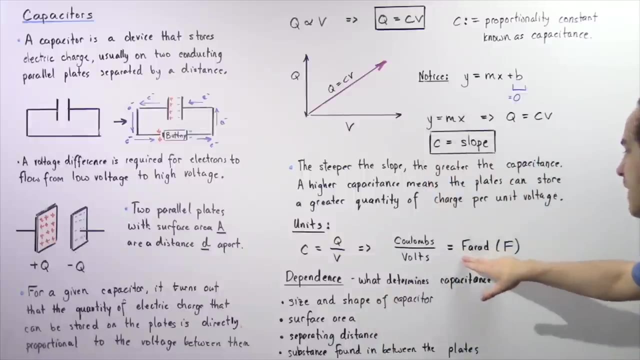 The capacitance given by c is equal to q divided by v, where q is the charge given in coulombs and v is the voltage difference given in volts. So we see the units for capacitance are coulombs per volts and this is given its own unit that is called the farad, given by an uppercase F. 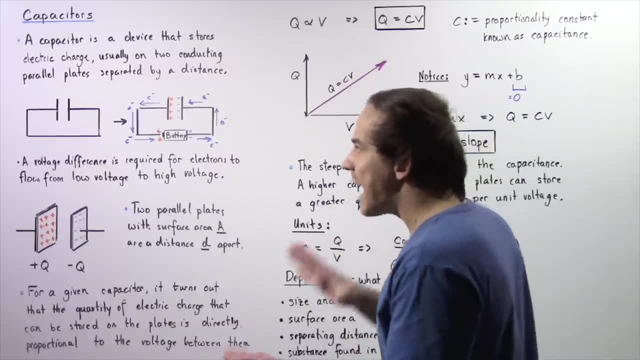 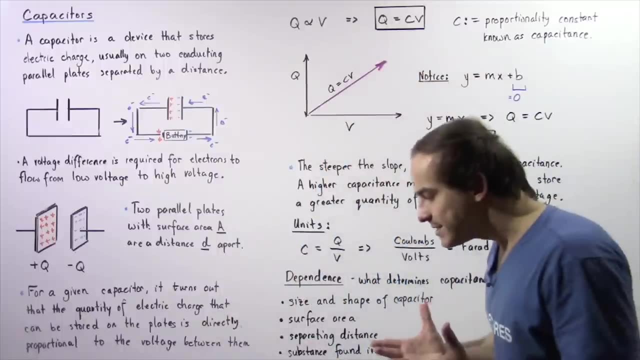 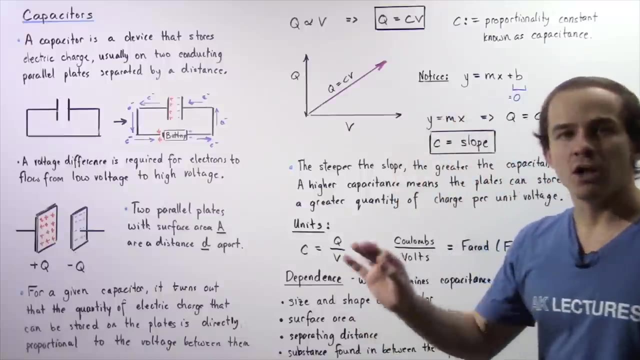 Now, what exactly does our capacitance depend on? Notice that, even though q is equal to c times v, capacitance doesn't actually depend on the voltage or the charge. Capacitance depends on other things that we'll talk about in a future lecture, But for now we'll mention that. 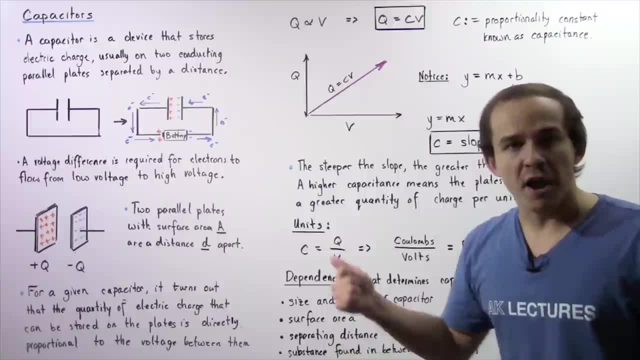 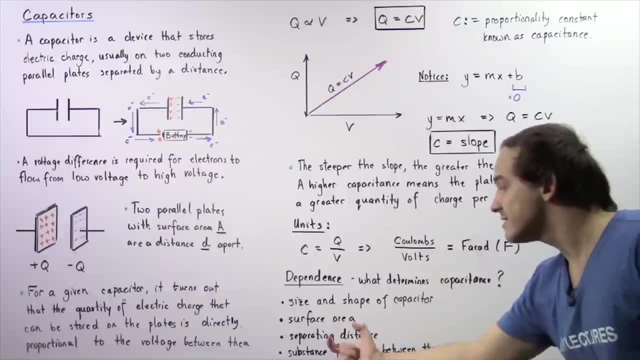 capacitance depends on size and shape of our capacitor, It depends on the surface area of the capacitor given by a, It depends on the separating distance between our two parallel plates, And it also depends on the distance between our two parallel plates. And it also 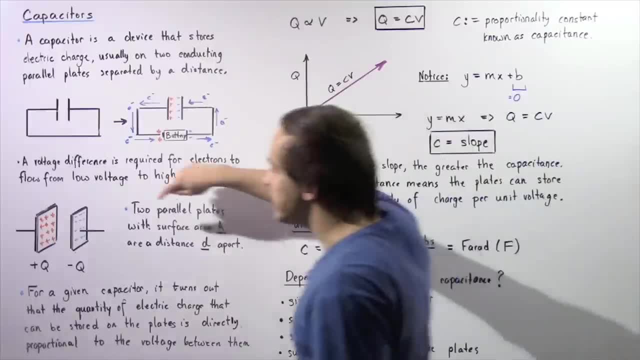 depends on the substance that is found in between our two plates. Usually, the substance is air.